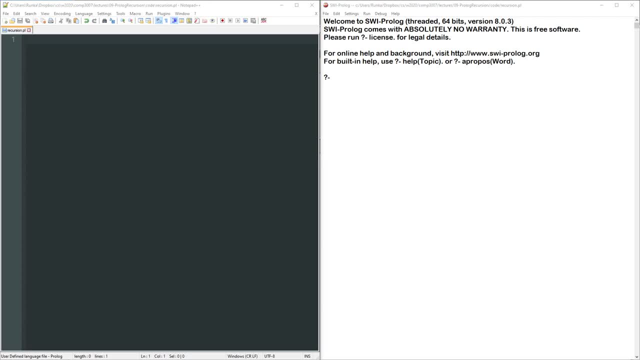 recursion in Prolog works like recursion in a lot of other languages. We have two parts. we have a base case and a recursive case. In Prolog these are typically represented as two separate clauses, a disjunction of two separate terms, where one represents the base case and another represents a 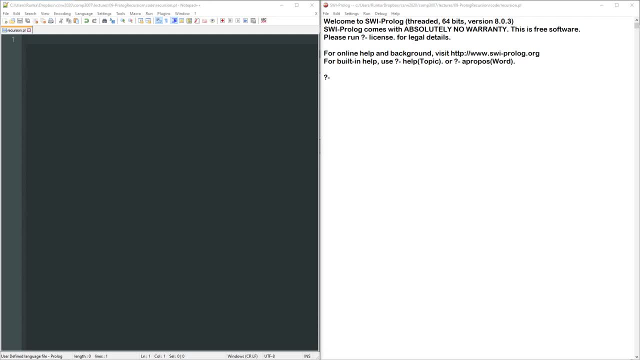 recursive case or a recursive rule. So consider, for example, summing a range of values between two integers, We'll say the sum, range function or some range rule from a, b and result. So it takes in three pieces of information. Takes in might be a bit of a misnomer. 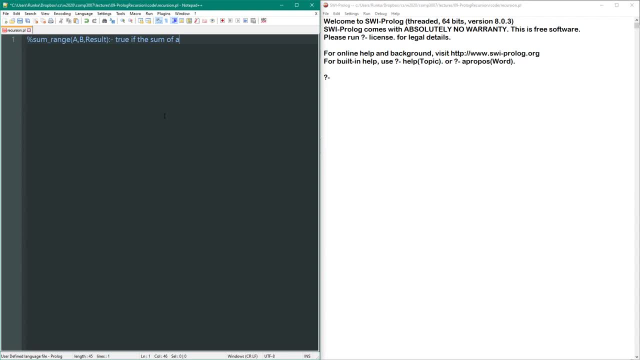 We'll say this is true if the sum of all the integers in the range from a to b is equal to result. This is a description of what this thing needs to be. Now, this needs to be recursive, Because we're going to solve it one piece at a time, because a and b might be. 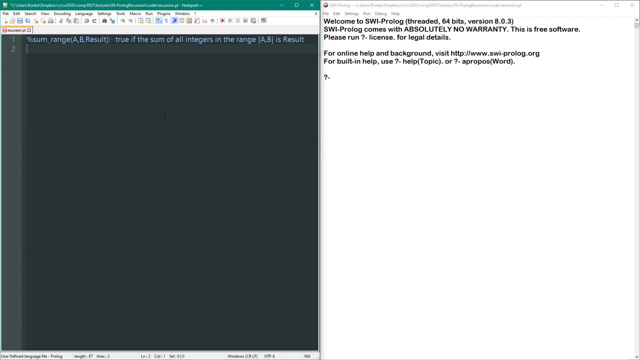 any different value. so we can't just explicitly code the, the summation, So we need to have some repetition in here. So we're going to need to have a base case and a recursive case. So the base case in this case is that a and b have reached. 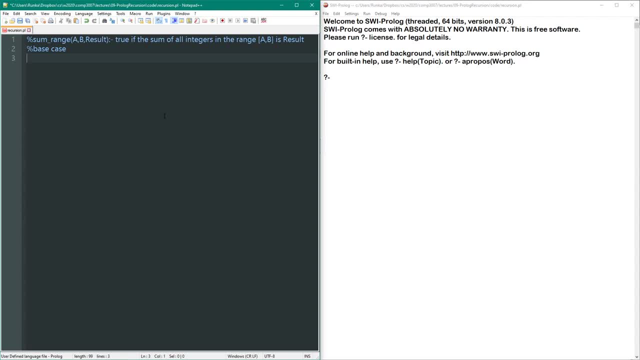 the same value. So for some range, like we saw it in scheme, a is the smaller of the two values. We'll assume that they're a is smaller and b is larger. Then a is just going to be growing each time through this recursive function. 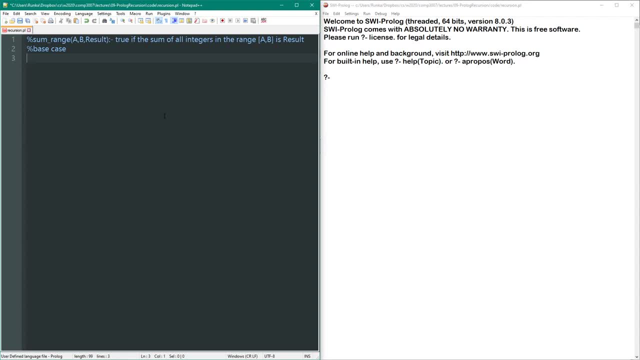 recursive clause and when it gets to this base case, then a equals b. So we'll say sum range with a, b and result, and this will be a rule. that's true if a is equal to b. Notice, I used double equals here. We don't want to unify them, We want. 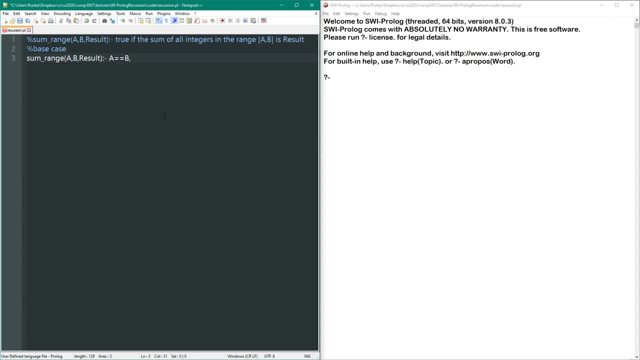 to say: if they already have the same value, that's great. Then this is the rule to be using. And then in that case we will say result and a should unify. Now, this will only work if the result variable is an unbound variable, and we'll see how all 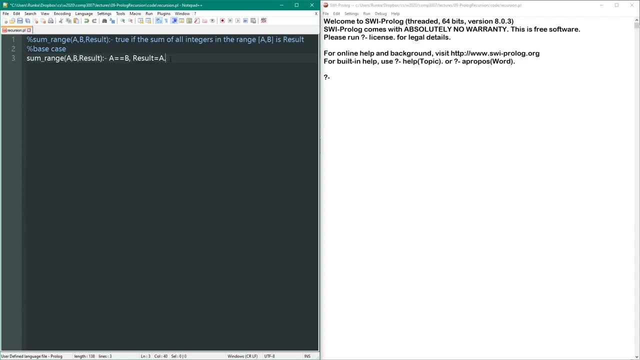 this pin sticks together once we see how the recursive case works as well. But the basic idea is, once we reach this case, we're going to take the result and store a value in it. And now our recursive case. So in our recursive case it's going to be a rule again. 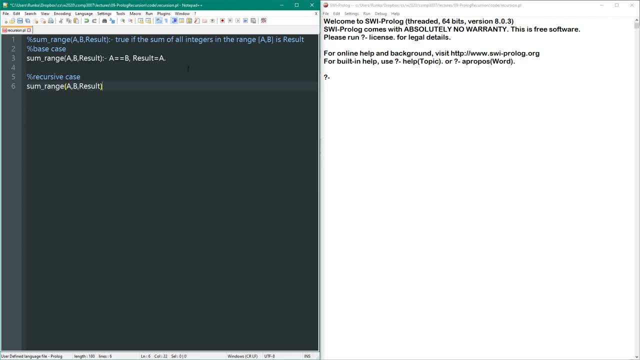 So we have some range a, b and result. Now notice, these two things have the same head. So we have some range a b result and some range a b result, which means they collectively, together define this predicate. some range, as we've seen it here. 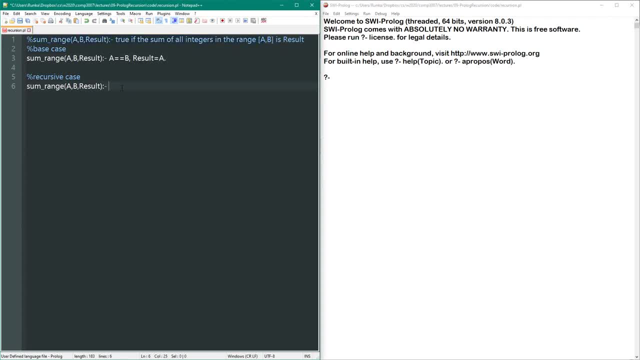 So we need both the base case and a recursive case, Two separate rules that together collectively define one predicate. Now for the recursive case. What we're going to do is add one value from this range into not so much a running total. we're going to do it with a recursive pattern as well. 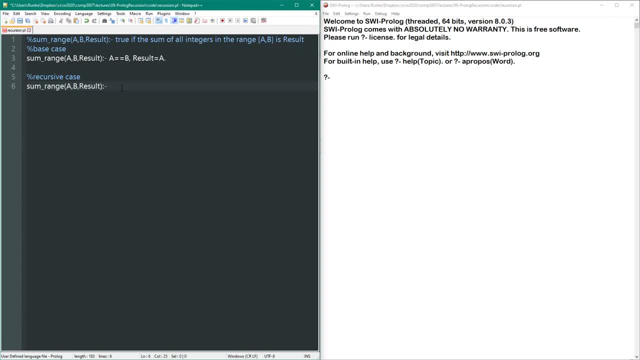 So we're going to defer the sum of one value into the result of adding up the rest. So we'll say the sum from one to ten is one plus the sum of two to ten, And the sum from two to ten is two plus the sum from three to ten. 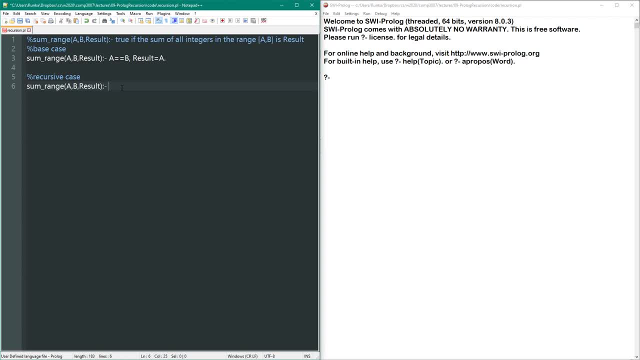 So to do that, we're going to have to get a few things. We're going to have to. We're going to have to increment our starting value. So something like a one is a plus one. This might seem odd, but we'll discuss that again in just a second. 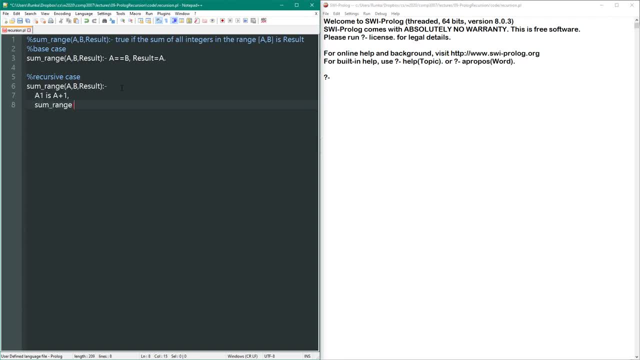 Then we're going to have a recursive call, So some range with that new value. So we've incremented a little bit And same value for b. B won't change in all of these And results Result. Now we don't want this to be the same result as this one up here. 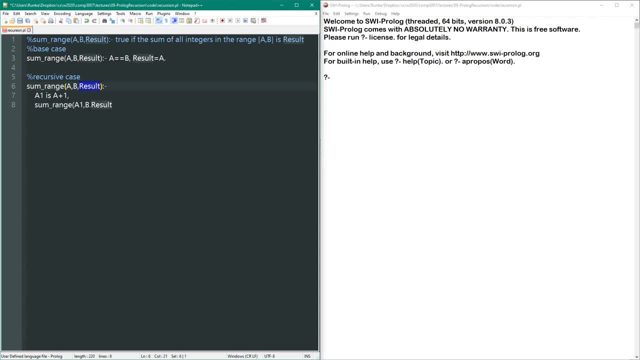 This is going to be the final result of this call. So this is the result of everything from, let's say, two to ten. Right, If we're passing in one to ten. A1 now has the value two, So it's a plus one. 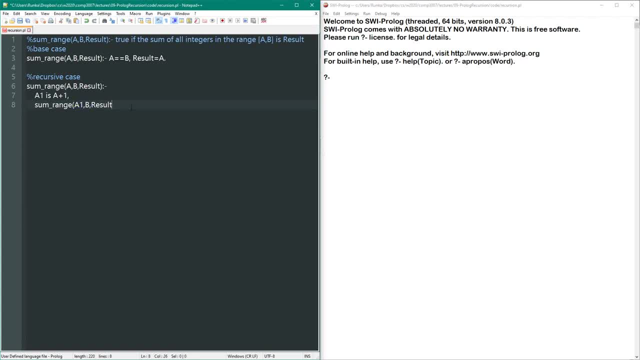 So this is the sum from two to ten. So this should be a different result, The temporary result. So we'll call it result1.. In terms of temporary result. And now what we need to do is take that temporary result And add the current value of a to get the total result. 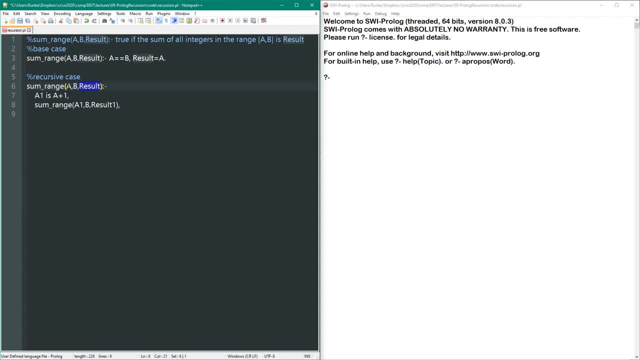 Right Again if we said: Uh, Um, one to 10 is one plus the sum from two to 10.. This is the sum from two to 10.. So now I have to add that one plus part and put it into this variable. 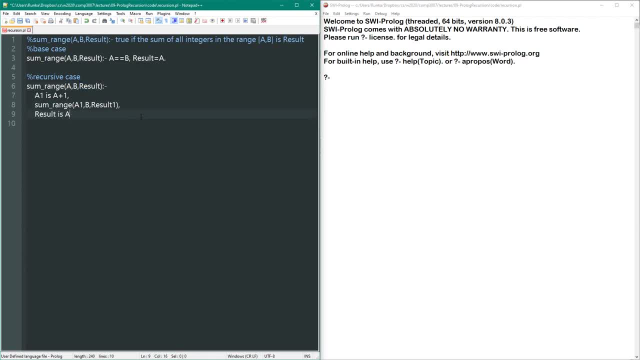 So we'll say: result is a plus, result one. Okay, so this is the sum from two to 10.. We'll add one onto that. Now we have the sum from one to 10.. Now, how does this all work together? 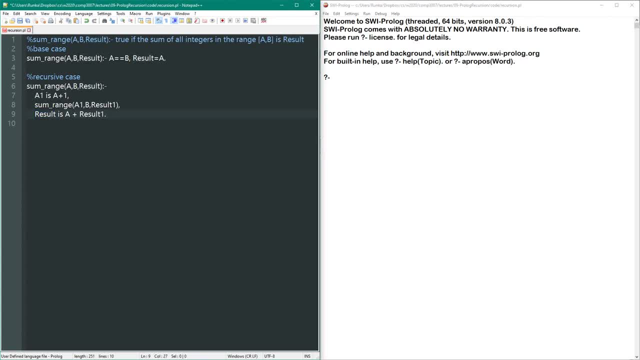 So this works a lot similarly to our recursive programming in Scheme. So we have a recursive case here, We have some deferred work, We have to do the addition after we do our recursive call. So starting from, let's say, one and 10 again, 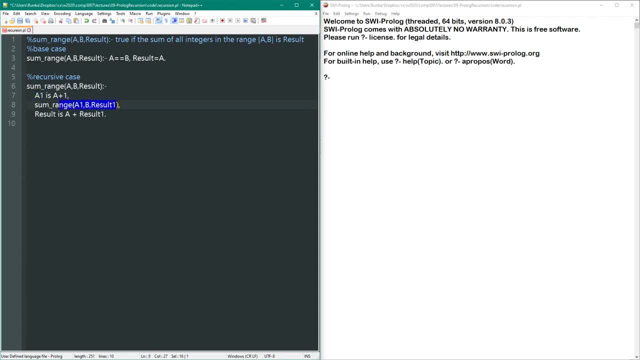 we say, well, a one is two, and we say, get the sum from two to 10.. And that comes back to the top and says, okay, from two to 10, a one is three, get the sum from three to 10.. 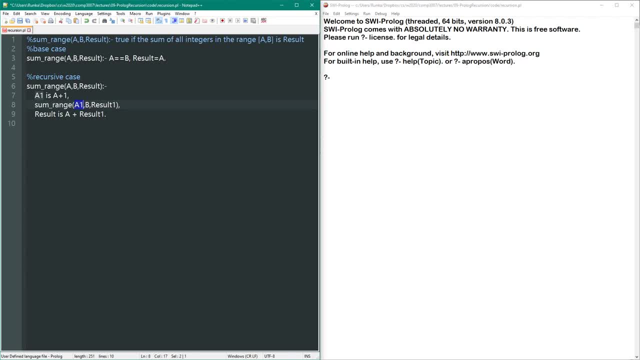 Get the sum from four to 10,, five to 10,, six to 10,, seven to 10,, all the way up. Eventually we get the sum from 10 to 10.. That reaches our base case. So a equals b 10 and 10, that's great. 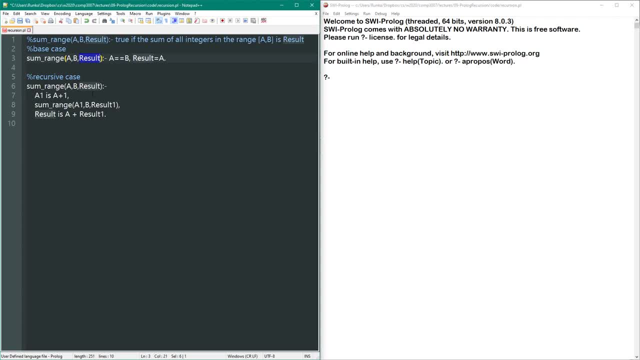 And then we'll say: oh, we'll say: result: this variable here that we haven't yet come up with a value for right. Each time we're passing in two: 10, empty variable. three: 10, empty variable. 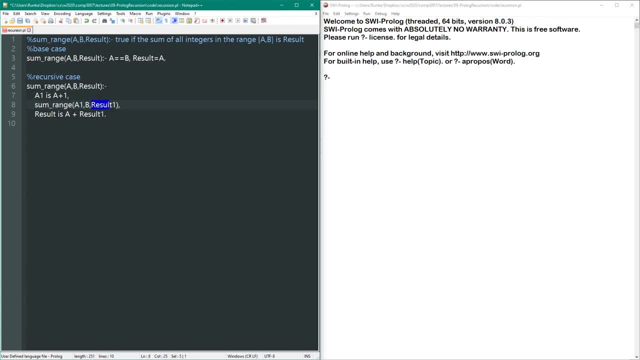 It's a different empty variable each time, but it's an empty variable. So we get to here we have 10,, 10, and an empty variable And we say put the value 10 into that empty variable. So that comes back to here and says: 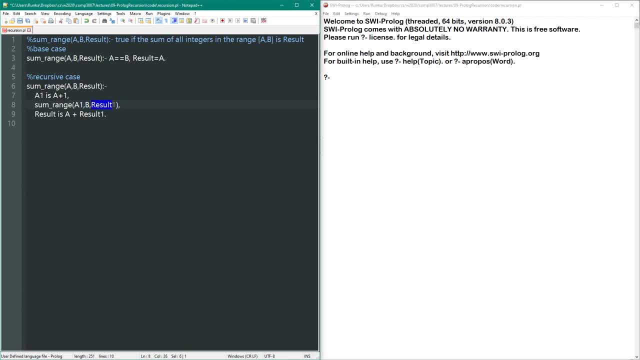 when I asked what's the sum from 10 to 10, it comes back with 10, great. So now we'll say: well, the sum from nine to 10 is nine plus 10. And we'll store that in result. 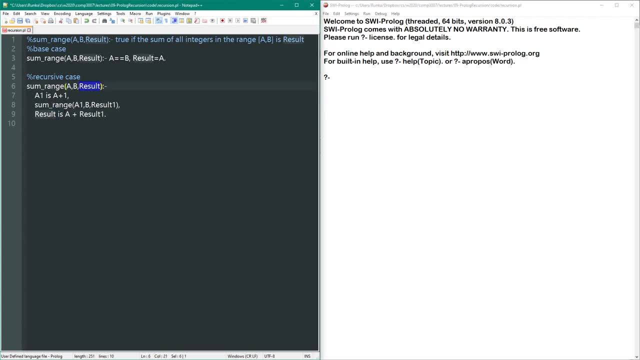 So that gets returned back through here. So then that comes back to where it was called from, where here we said: sum the values from eight to 10.. And that was nine plus 10, which is 19.. So result one is 19.. 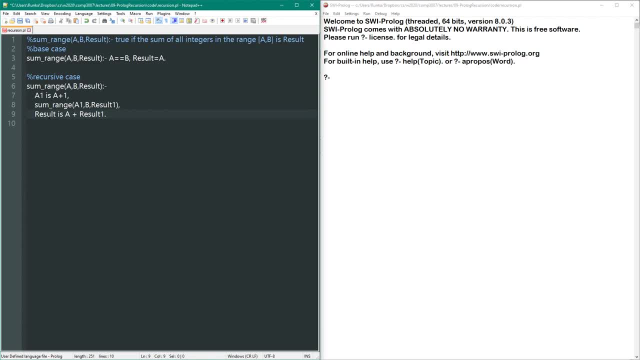 And we say, well, add eight onto that 19 to get 27.. On and on and on all the way back down, And eventually we'll have all the answers. sorry, eventually we have all the answers. back to our query. 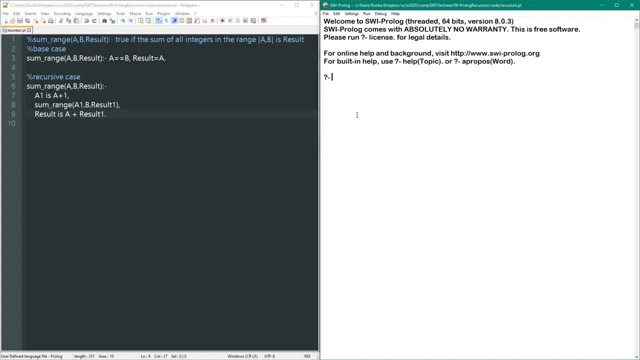 So let's try this out. Sure, let's just query this then. So sum range from one to 10, R. So notice, when I'm querying this I'm providing values for the information that I know I want to have 1 and 10.. 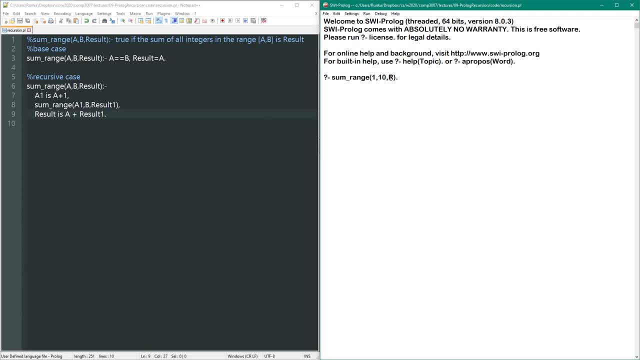 That's the range of inputs, And then this last one here is left as a variable, a lot like when we were doing queries before, when we weren't doing any repetition or anything. We left an empty variable, for example for our coffee manager thing. 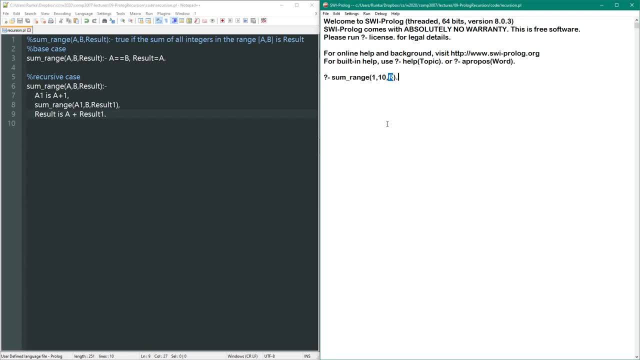 We said manager X, And that's true if X is Bob. This is the same sort of idea, except there's going to be more steps going on, So they're going to create a linkage of all of these results where result equals A plus result one. 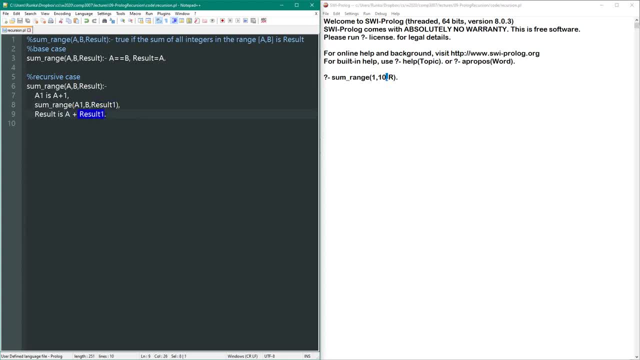 And result one equals A plus a different instance of result one, And it goes all the way down until eventually this unifies with this And it actually gets its value at that base case. So we pass in actual values 1 and 10 for A and B and an empty variable for R. 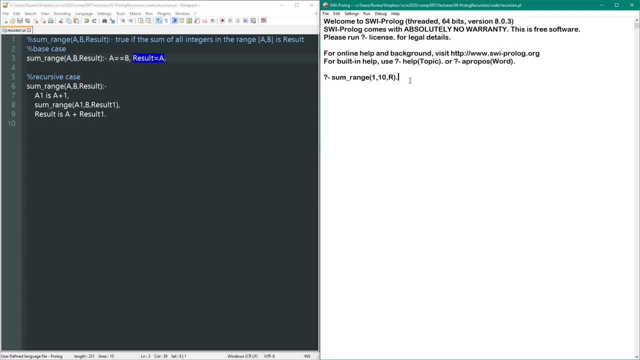 asking for an output variable. So you can think of that a little bit like a fishing hook or dropping in this empty variable. It's going to go through all this work. Eventually it's going to have a value put onto that hook And then when it comes back out through the recursion. 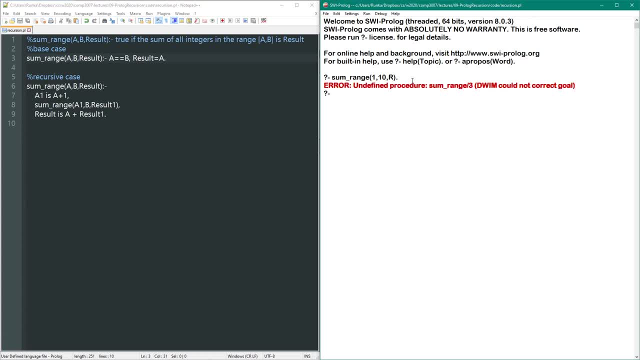 we'll have that value out in our query space Helps if we consult our knowledge base. So recursion and then try again. There we go. So the sum range- 1 to 10, is 55.. We can also ask a similar question. 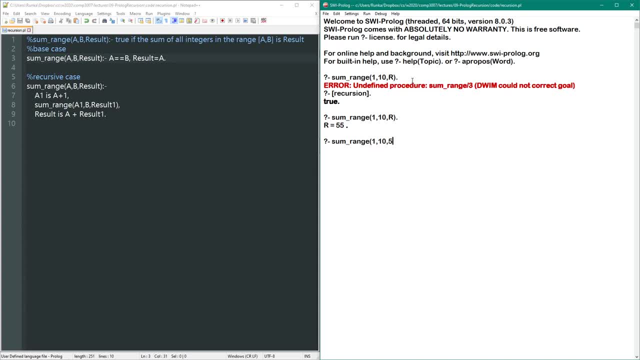 Is the sum range from 1 to 10 equal to 55? And that comes up true. We can do that for other values as well. So sum range from 1 to 100 should be 5,050, like that. Or I can put in a variable and see what it is. 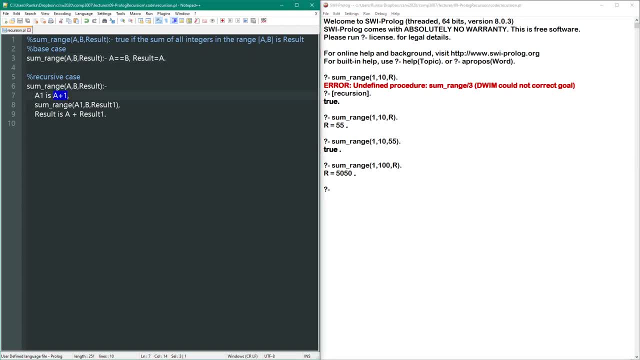 So we can do these reversible a little bit. We have some arithmetic in there. So for example, we can't pass in an unbound variable for a. Similarly here we can't pass in an unbound variable for b, because it's asking: does b have the same value as a? 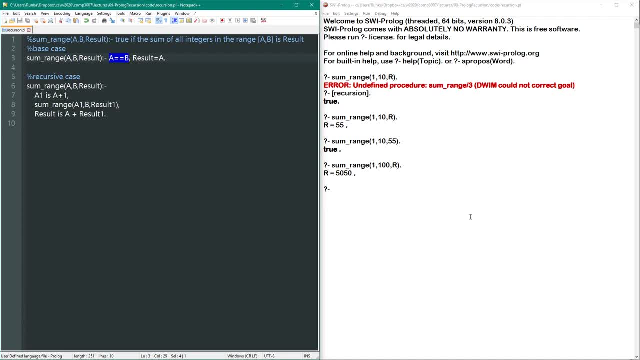 But for r we can either include a variable or not include a variable, And it will either return true or true with a value. OK. so a few other things about this code. As I mentioned before, this a1 is a plus 1. 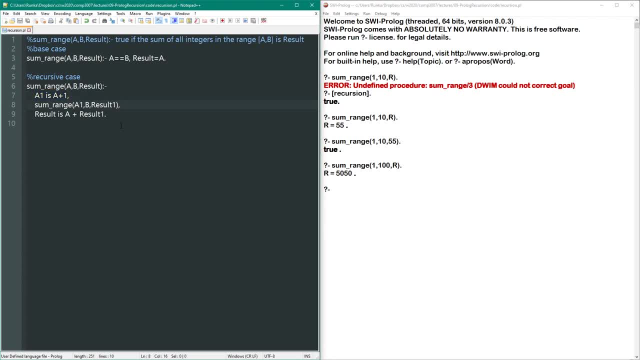 might seem a bit odd. Normally we do something like this, where we just say: call the function sum range with a plus 1, b and some sort of result variable. This is our output. Prolog doesn't let you do that. Prolog says you have to do all these steps individually. 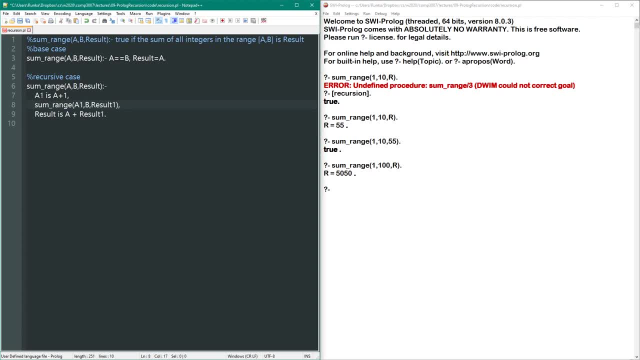 So we can't nest these in here. So we have to say: figure out what a plus 1 is and then pass that value into the next instance of our function. And one other thing to point out here: this base case, while effective, is not necessarily. 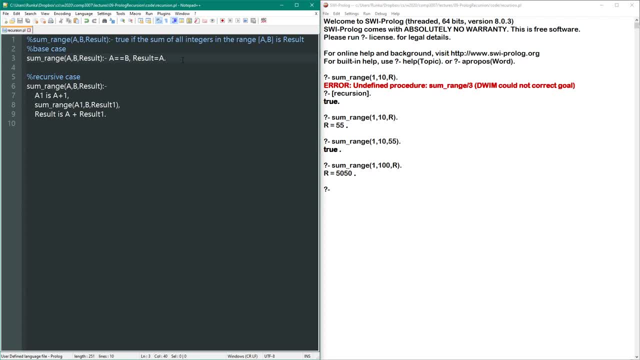 the most abbreviated. In fact, seeing base cases like this is a little less common. in Prolog You're more likely going to see something more like this. If you say sum range aaa, which seems really strange. right, With this first one, you can say: OK, we're. 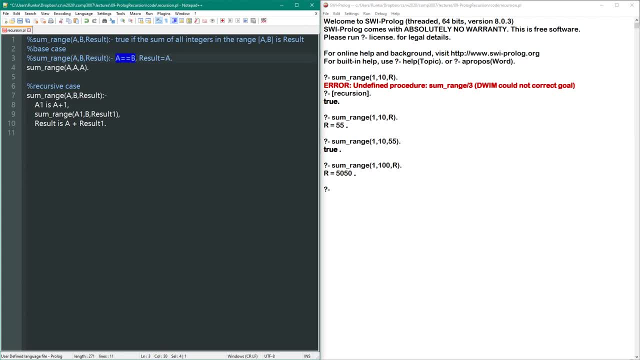 taking in two values, a and b, and an empty variable, result, And then if a is the same as b, then result gets the value of a. That looks a little bit more like an imperative program, but Prolog is not an imperative programming language. 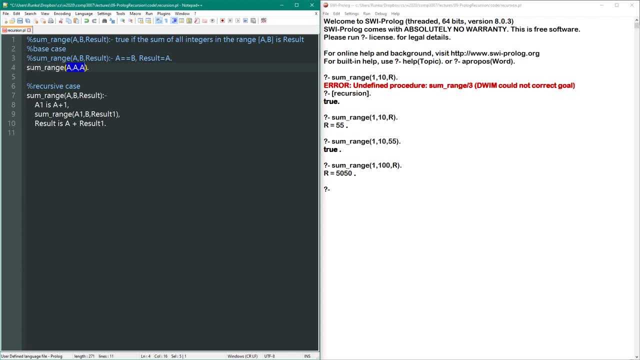 as we've seen. So what this actually says is this will unify with any situation where the first two values are the same and the third one's an unbound variable which now has that value right? So think, if I asked, sum range from 1 to 1 with r. 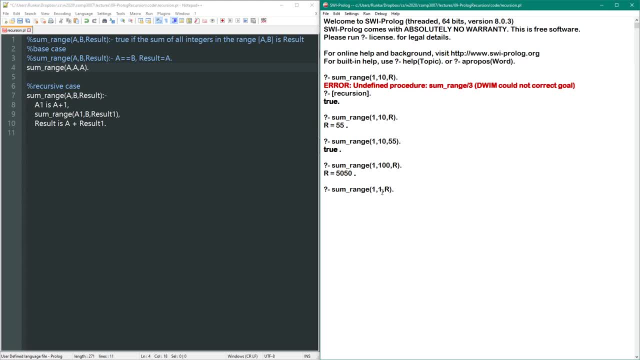 Well, what is the sum of all the integers between 1 and 1?? Well, it should be 1.. So this will unify with this fact because 1 and 1.. So we have essentially a situation where our start and end values are the same. 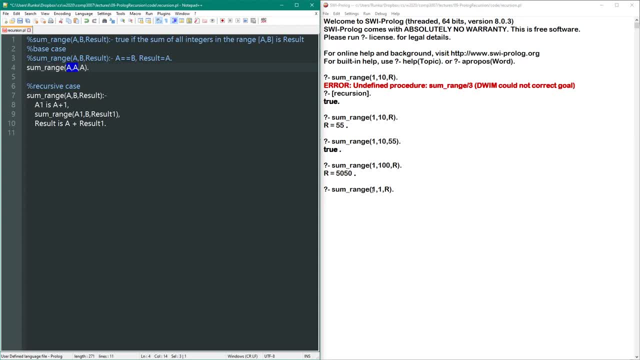 We just use the same variable in both those spots. And now, because that variable in this case is bound with the value 1, what happens when we use that variable as our result space here is that r will unify with a And these a's unify with 1.. 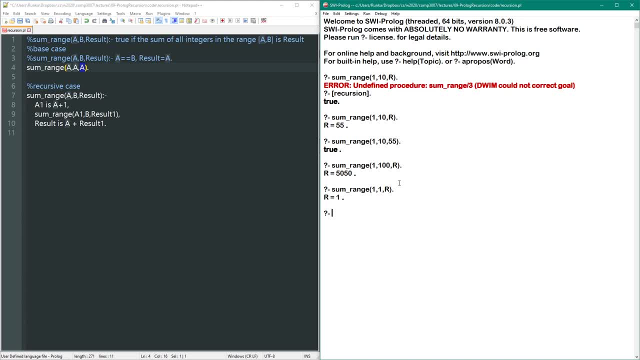 So r unifies with 1.. So it's a bit of an odd way of saying it. It's saying the exact same thing as this, just in a much more compacted notation. So it says: if these two things are the same. 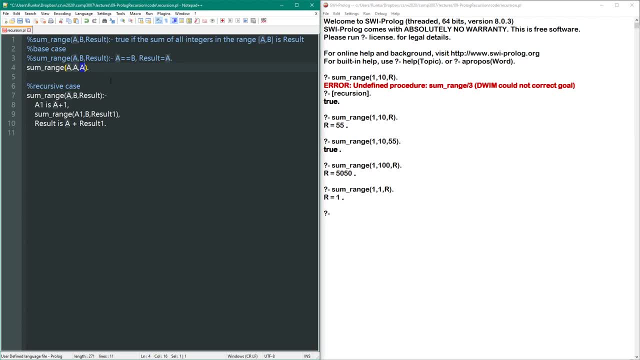 then take that value and put it here as well. So that's the idea behind recursion in Prolog. So we have a base case and recursive case, as before. The recursive case needs to Here. Sorry, Is dependent on a function call. we'll call it to that same rule. 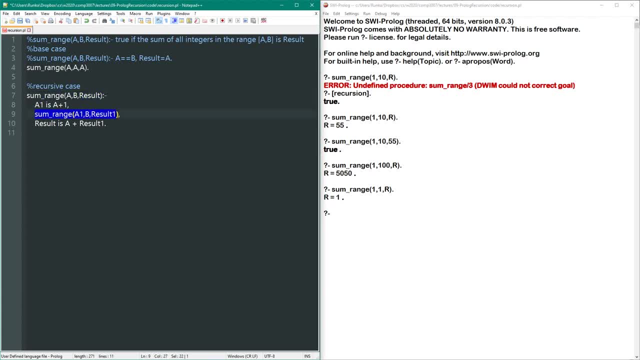 So this sum range is dependent on a different sum range And, as always with recursion, it's very important that something in that recursive case shrinks the problem so that we eventually reach the base case. Otherwise we end up in situations like we saw in the last lecture for the symmetric and transitive. 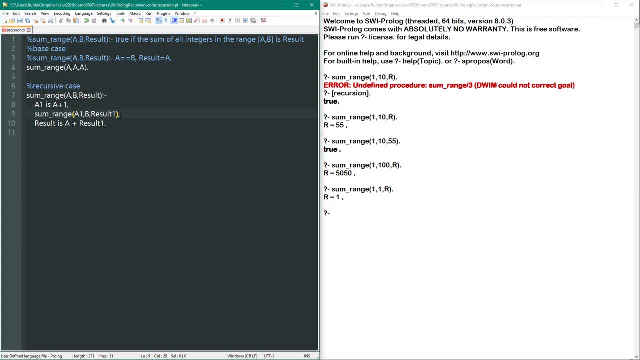 properties, where we had that infinite recursion because our problems weren't getting any smaller. OK, Let's do another example. Let's do the Fibonacci sequence, So fib, Oh, hang on. I never actually tested this new version of recursion. 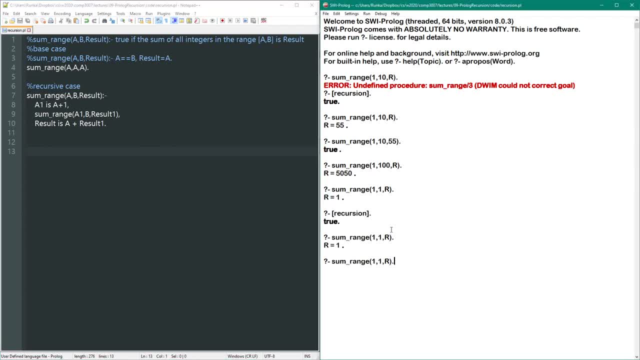 Just to demonstrate that it actually works. There's the same thing. OK, Now I wanted to show the Fibonacci sequence, So let's do that next. So fib of 0 is 0.. Fib of 1 is 1.. And otherwise the Fib of n is equal to the Fib of n minus 1. 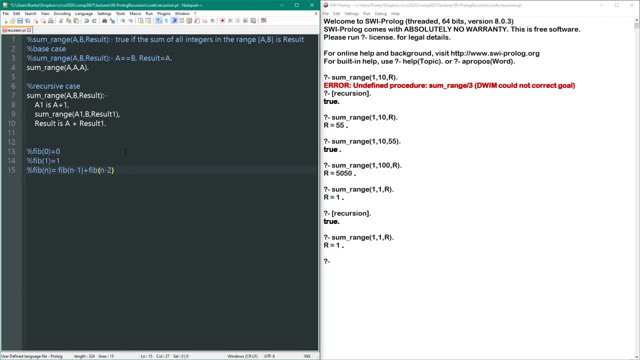 plus the Fib of n minus 2.. We've seen this example a number of times. It's most useful, at least in computer science, as I've seen it as an example for demonstrating branching recursion. So let's see what happens if we want. 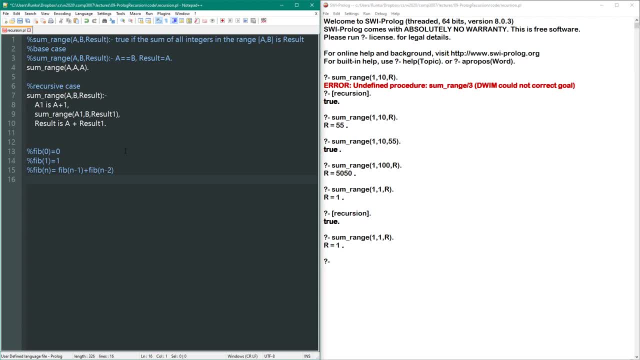 to code this example in Prolog, So We have to get this. OK, Let's deal with our base cases and our recursive cases. Now, as it turns out, we have a pretty simple definition of a recursive program here. So our base cases. 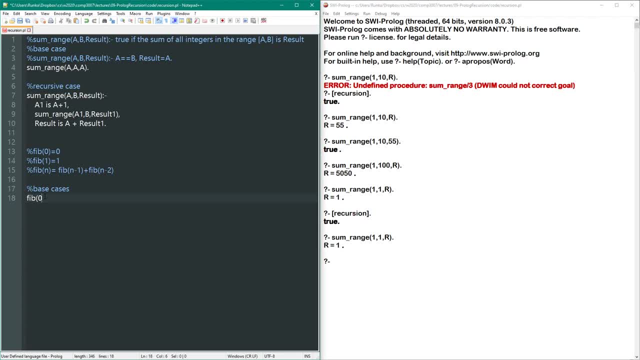 In this case, we have fib of 0. So fib of 0 is 0. And we have fib of 1, which is 1.. So the way to read these is: this is our input. The first value is our input. 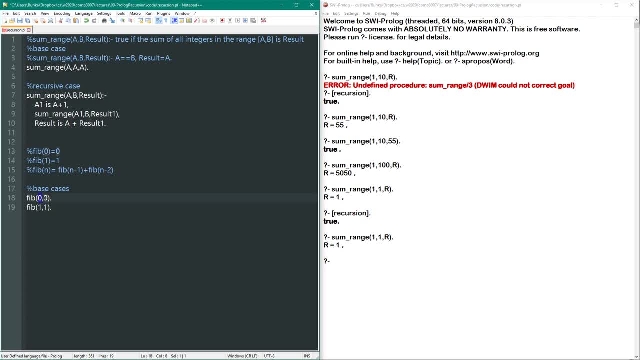 And the second value here is our output. So if we're given a 0, we'll return a 0.. If we're given a 1, we'll return a 1.. So when calling this, if you want to know what the nth Fibonacci number is, 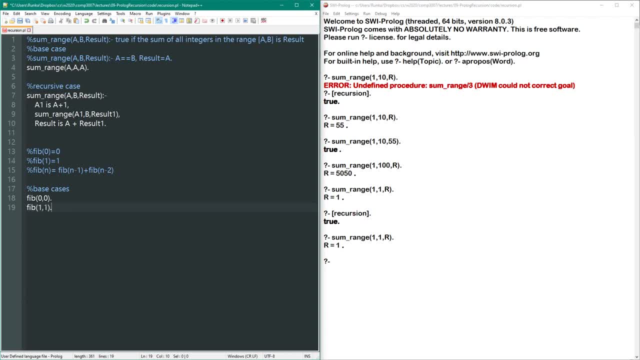 let's say, if we want to know what fib 0 is, we'd say fib 1, x, And that says that's true if x equals 1.. That's how we know that the value of the first Fibonacci number equals 1.. 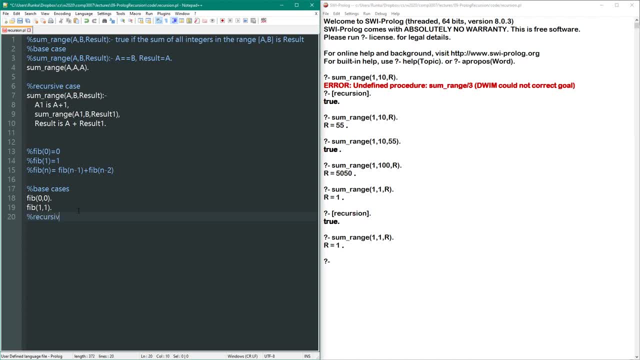 Now for our recursive cases. it's a little bit more involved, But it's no different than what we've seen before. So for the recursive case we need to calculate n minus 1 and n minus 2.. Evaluate Fibonacci on those n minus 1 and n minus 2s. 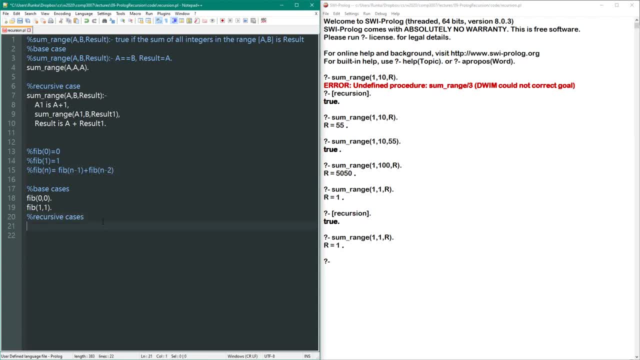 And then add everything together to get fib of n. So we get a rule for this. So we'll say fib of n is r. So again, the way to read this is the nth Fibonacci number is the value r. So if somebody is requesting this, they'd say fib of 10 is x. 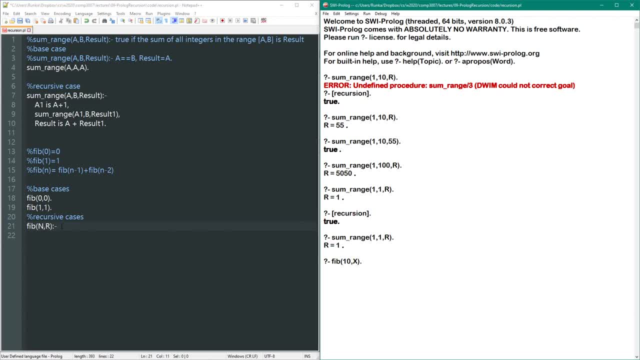 So x unifies with r. So in the end whatever answer we put into this variable r in our rule will go out into the query as x. But then whatever value the user puts into, n is the value we need to work with to create our answer. 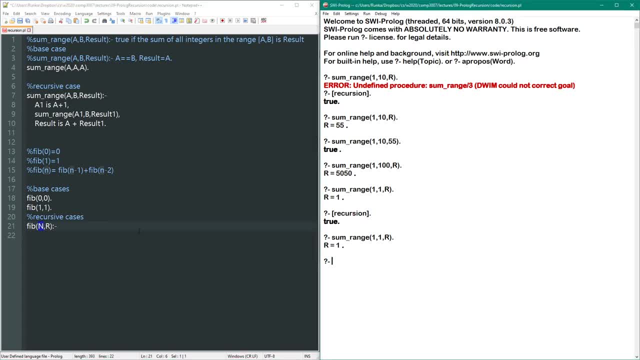 That's not going to work because I haven't reconsulted this yet, So let's just delete this for now And let's create our rule. So first things first, we need n minus 1 and n minus 2.. As we saw in the previous example. 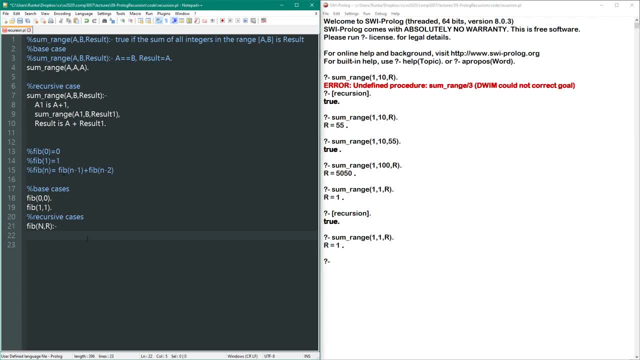 we can't just do that inline, nested inside the Fibonacci call. We have to do that first. So we'll say n1 is n minus 1.. And notice, you can't say n1 equals. We've said it. We've said it. 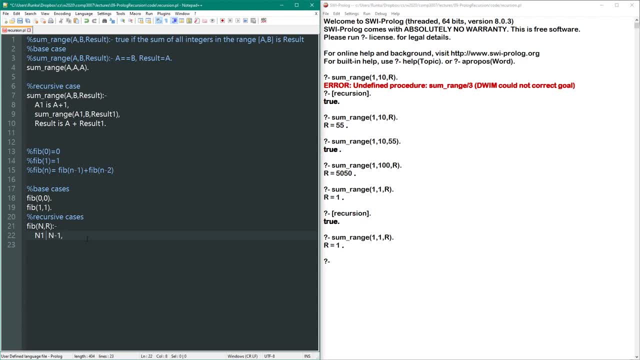 We've said it, We've seen this before: If you want the arithmetic to actually take place, to actually be evaluated, you have to say is, So is says, evaluate this expression and then unify it with this unbound variable. We have n2, is and then n minus 2.. 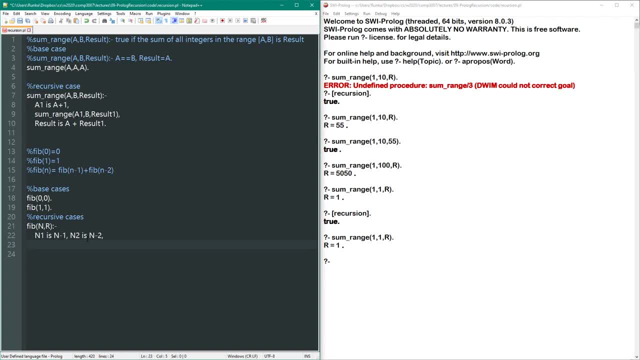 In fact we can do those on one line there, just to keep our code a little bit compact. The next thing is: we want to calculate the fib of n1 and the fib of n2.. So we can say: fib of n1 is r1 and fib. 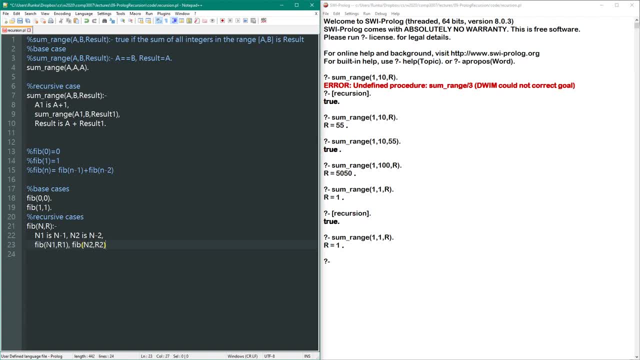 of n2 is r2.. So we call Fibonacci on this n minus 1 value and on this n minus 2 value And we'll get back values r1 and r2 that represent the n minus 1 and the n minus 2 Fibonacci number. 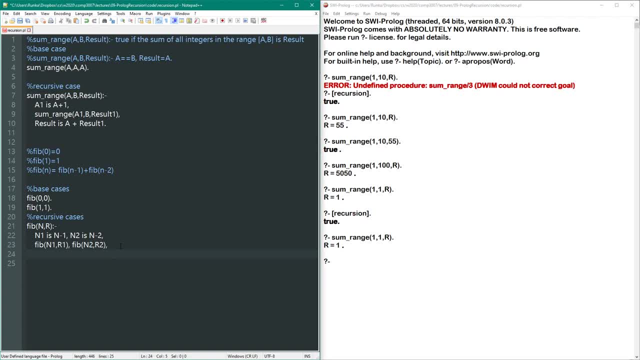 OK, Now all we need to do is take those two results and combine them together into our final result. So our final result needs to be put into this variable in the end, because the user, as I said before, is going to type something like fib10 of x. 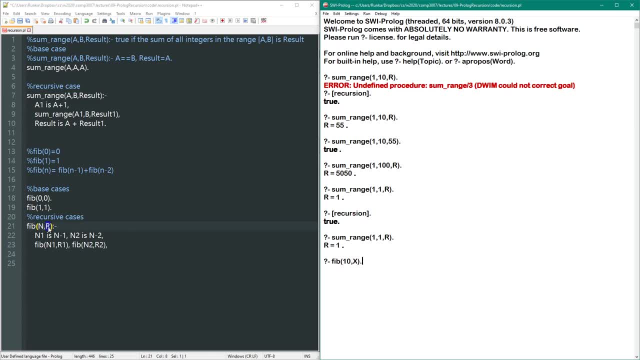 X is going to get unified with r. So whatever value we put into r is going to get put into x. So we would say r is r1 plus r2.. These two things should have numbers based on the previous lines. So we call fib of n1 to get the values for r1 and r2.. 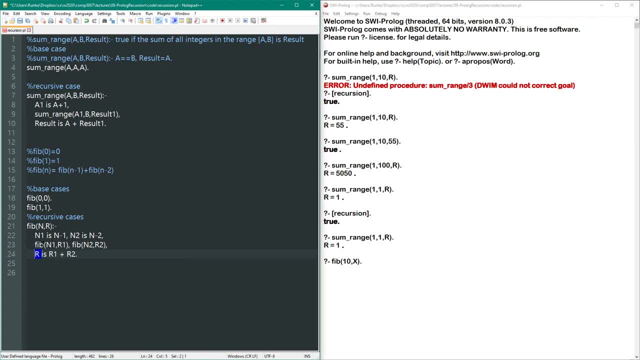 So we'll just add those two values together to get the fib of n. OK, So that's this one here And that goes back to the user, And we're done, Do, do, do, save and reconsult. OK. 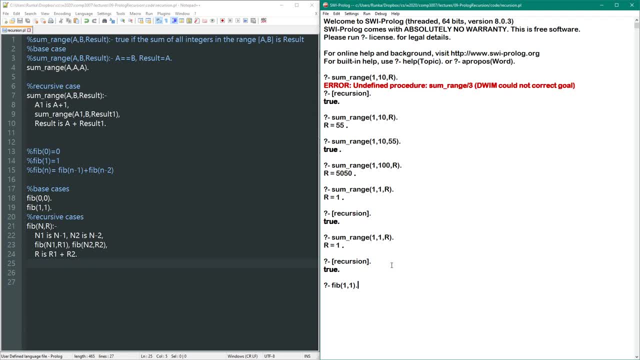 So we can say fib of 1 is 1, right? So for example, we can just run this where we pass in both our inputs and our outputs and sort of verify information that we think we know. So if we run fib of 1, 1, we just get true in that case. 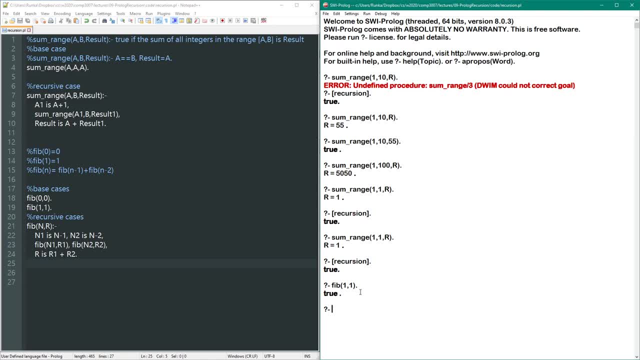 So it verifies our intuition. Alternatively, we could ask: what is the value of these things? We could say: fib of, let's say, 7 is x. Now 7 goes into n, x unifies with r And it walks through this whole recursion. 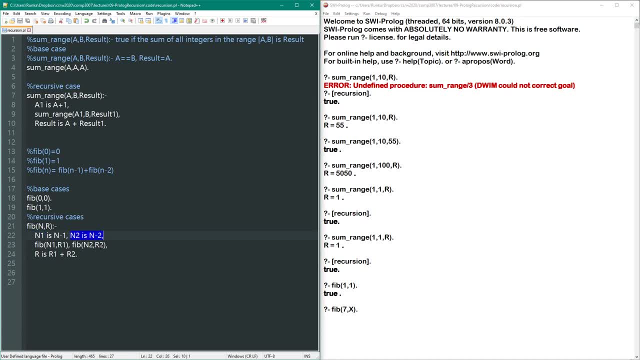 So n1 becomes 6.. n2 becomes 5, 7 minus 2. And it queries fib of 5 and fib of 7.. Now, not walking through the entire tree, but those will come back with values for fib of 5 and fib. 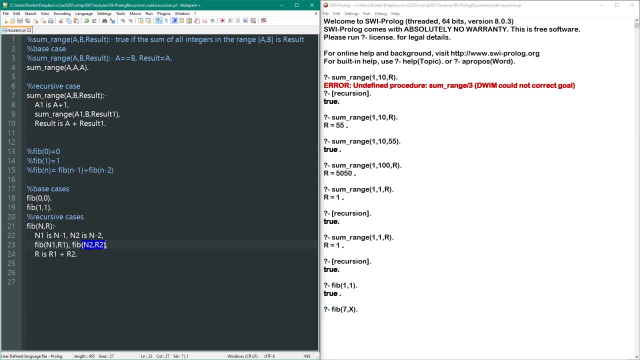 of 4,- sorry- 6 and 5.. I can do math, OK. OK, So fib of 6,, fib of 5. And we'll have values for those And we'll just add them together to get the value for fib of 7.. 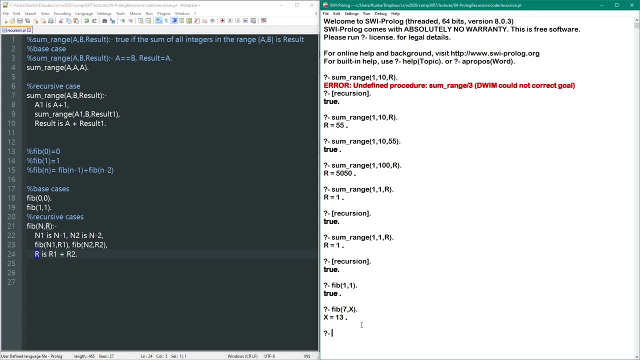 There we go, 13.. Right, That's basically it there Now. there's a few things to notice about recursion in Prolog, though. First off is that order is very important. So, for example, what would happen if we rearranged? 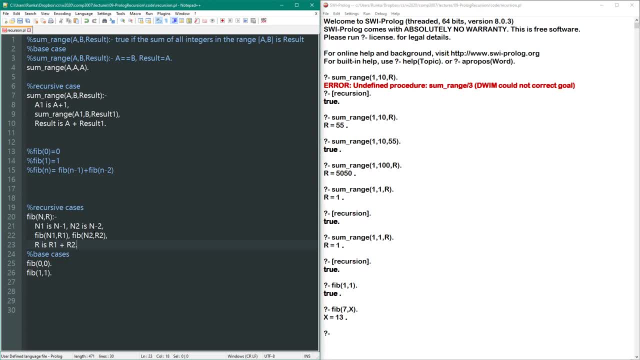 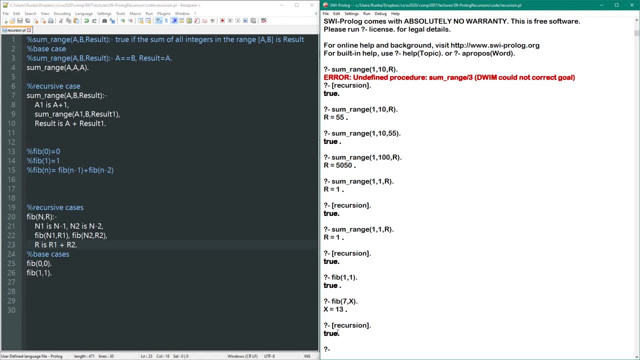 the order of our base cases and our recursive cases. So I save this and reconsult recursion. So just pause for a second and think what would happen. What would happen if I queried, for example, fib 5r? Well, let's run it and see. 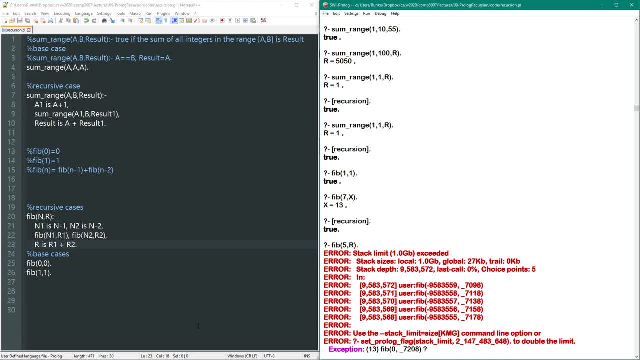 Oof, the whole thing crashes, Stack, limit exceeded And you can see the error was many calls to fib with some weird numbers. All right, All right. The issue here: we said fib of 5, which then asks: well, create 4 and 3 as n1 and n2, and then call fib of 4.. 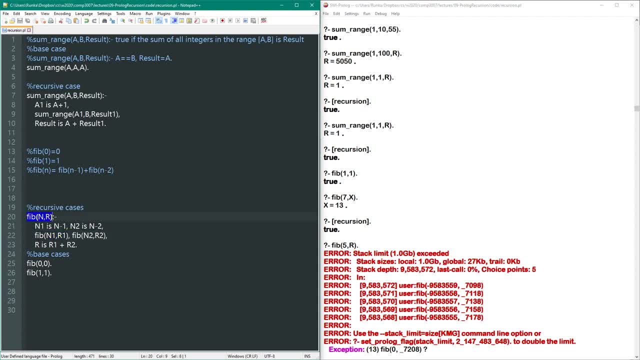 It comes back up And that's going to match with the head of our rule. So 4 makes it 3.. Call fib 3.. And then 3 makes this 2.. So call fib 2.. And then this is 2.. 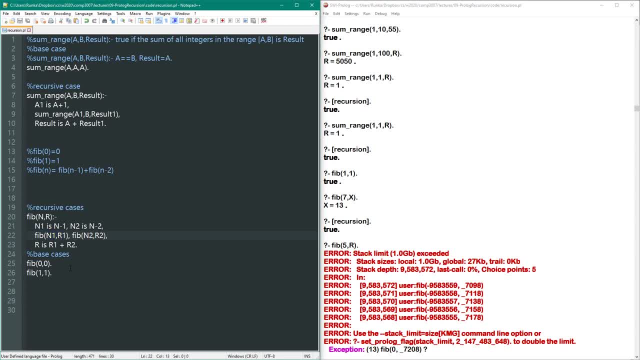 So that makes this 1.. So call fib 1.. And notice, when we call fib 1, we start at the top still And we match that with our rule. So that makes this 0. And we call fib 0.. 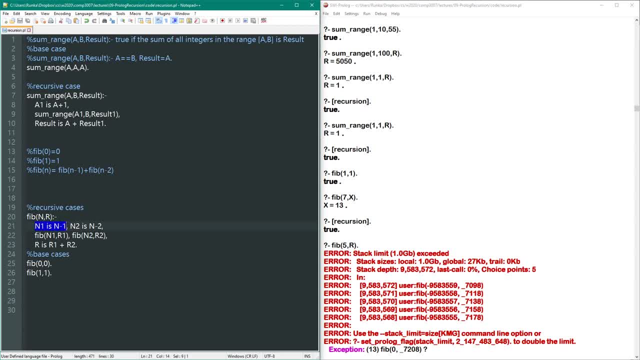 And even then we match with our rule. So we get fib negative 1.. And we call fib negative 1.. And again, and again, and again. The issue is we're always hitting this recursive case first. We're not asking: is it one of the base cases? 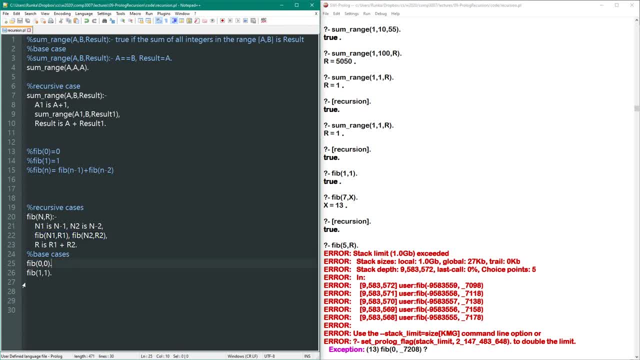 If so, stop, And if not, then do the recursive case. We're saying: just do this recursive case every time. It never actually finds these base cases. So So the stack fills up with all these recursive cases And our code fails. 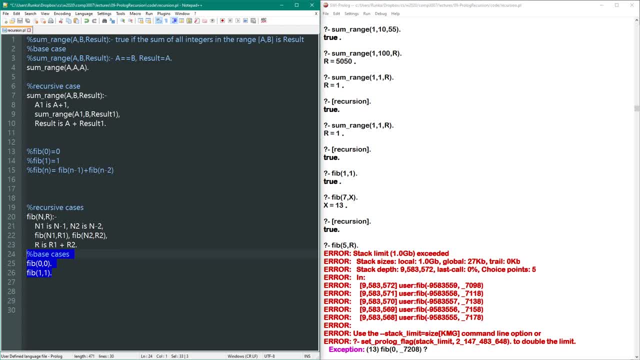 So order is important And, generally speaking, the base cases need to be put first, And this is true in Scheme as well. If you have, for example, a cond statement, you'd have your base cases first And then in the. else would be the actual recursion. 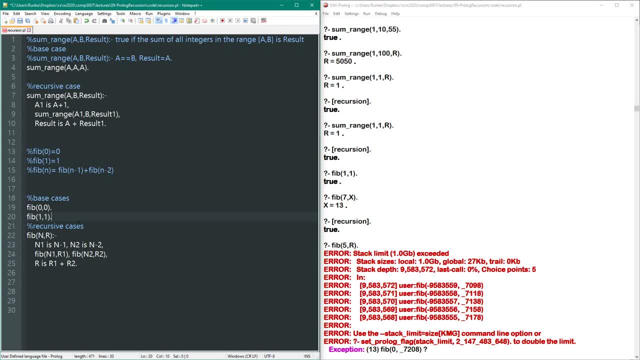 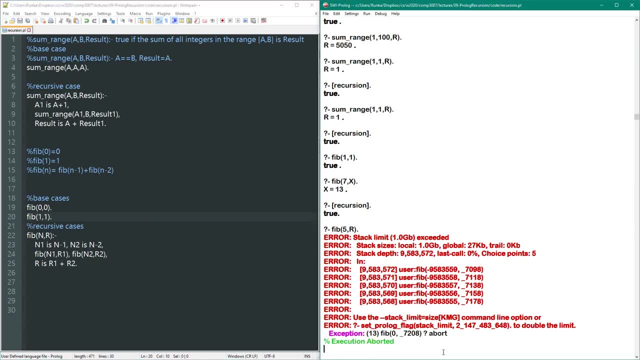 You're not going to just recurse and then check. oh, should I have stopped earlier, All right. One other thing to note here is: if I run this same thing, So let's save abort, Reconsult And let's ask fib5r again, since it's here. 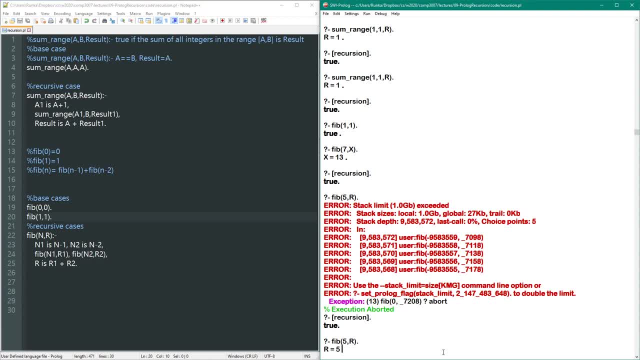 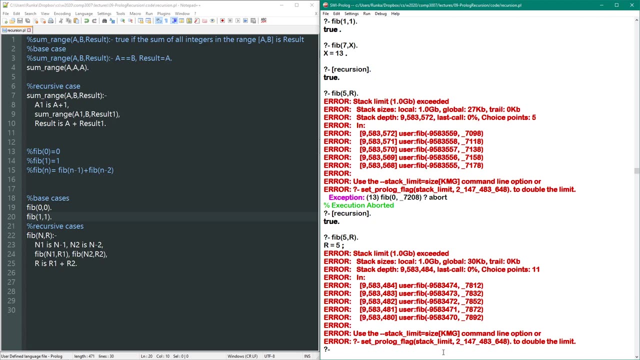 I get r equals 5,, which is true because it's 1,, 1,, 2,, 3, and then 5.. It's the fifth Fibonacci number. What happens if I backtrack here? We get a very similar looking error. 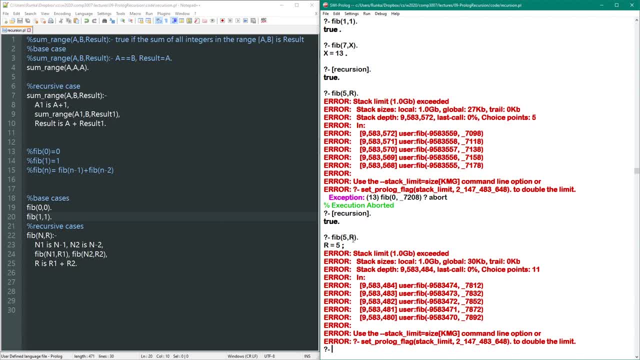 The reason here is pretty similar as before. So the success here: fib5r returns 5, is true because eventually, when we're calling these Fibonacci, these smaller Fibonacci's, we're eventually going to hit these base cases Now at some point. so sorry, we hit these base cases. 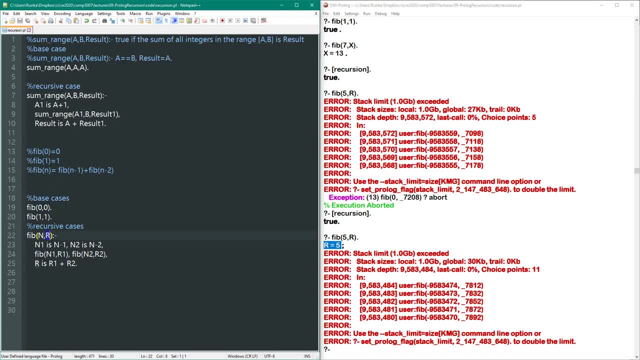 and it's going to return back up the call stack with all these unifications, where r is the sum of the two previous r's And then we get our value, that r equals 5.. But if we put in a semicolon we're saying well. 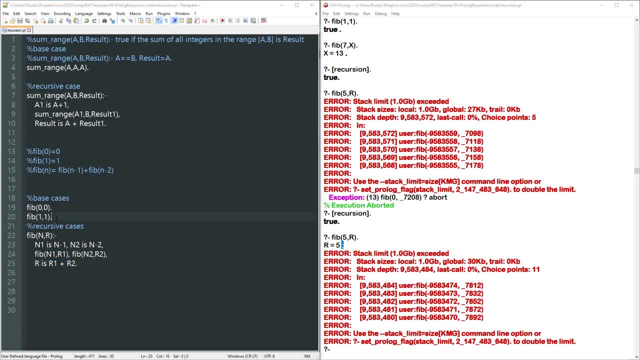 backtrack that, Try something else. So what that's going to do is going to take one of the situations where I hit this, the base case, and say, well, what else could we have done with that? So if it unified fib as one of the base cases. 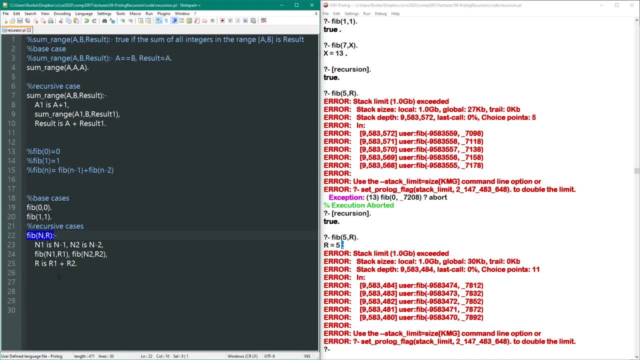 that's going to backtrack and say, well, I could also satisfy that by using this rule. So a fib then has 0. And 0 also calls negative or sorry, fib calls fib of 0 and fib of negative 1.. 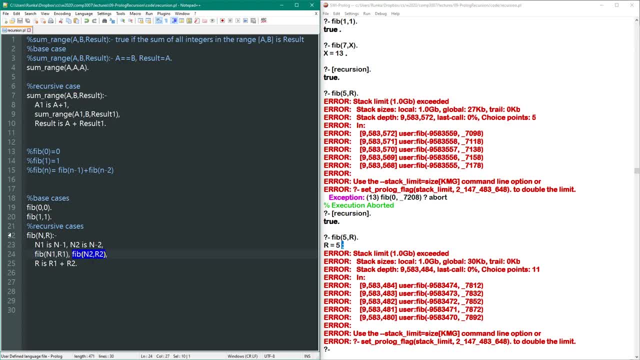 fib of negative 1,, as we've seen in the previous example, will then not match our base cases and go right to the rule: Negative 1 gives us negative 2 and negative 3.. Negative 2 gives negative 3 and negative 4, again and again. 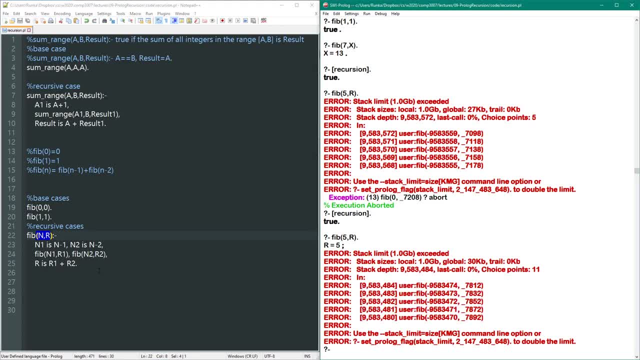 for infinity, where we have then a full call stack. So the way to fix this specific problem is to just be a bit more specific in our recursive case. So our base cases are true for these two very specific values, 0 and 1.. 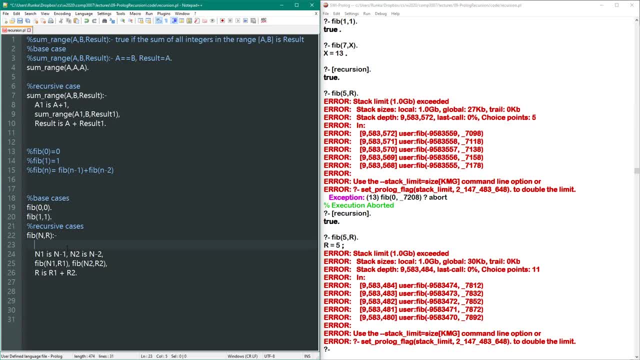 So our recursive case should only ever apply to the other values. Right now, they also apply to 0 and 1.. So what we should say is: well, I'm going to call this 0. Only use this recursive case if n is strictly greater than 1.. 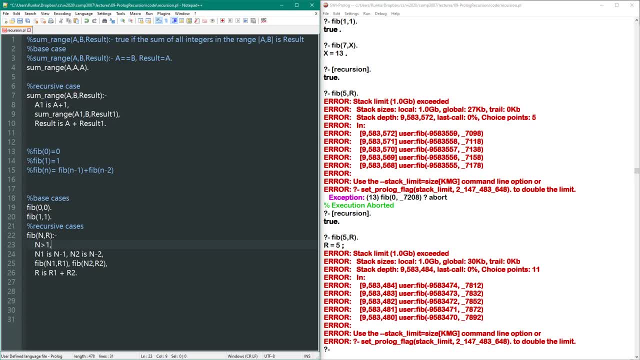 If it's a negative number, just ignore it. There's no such thing as a negative Fibonacci number. If it's 0 or 1, only use the base case. Never backtrack and land on this recursive case. Save, reconsult. try it again. 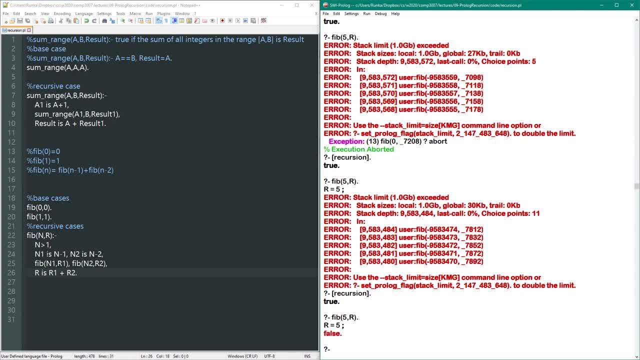 There's our success. And if we try to backtrack now, it lands on this recursive case: sees that n is not greater than 1, because n was bound to one of these base cases originally, That backtracked into here where n was, let's say, 1 or 0,. 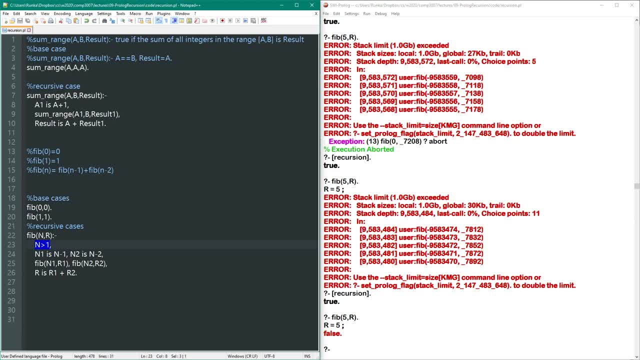 possibly, And neither of those are going to pass this test, So it then says false. There's no other values for Fib 5.. All right, So I think that covers our recursive introduction video. In the next video we'll take a look at recursion and iteration. in Prologue. 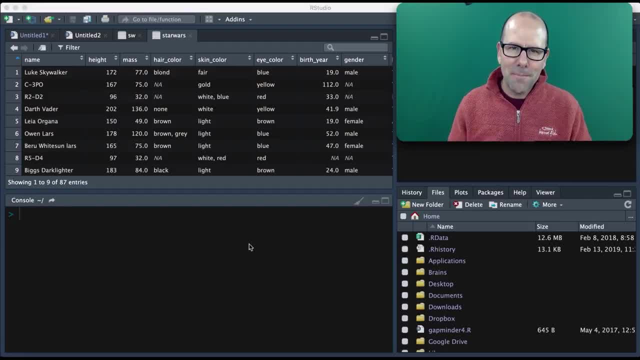 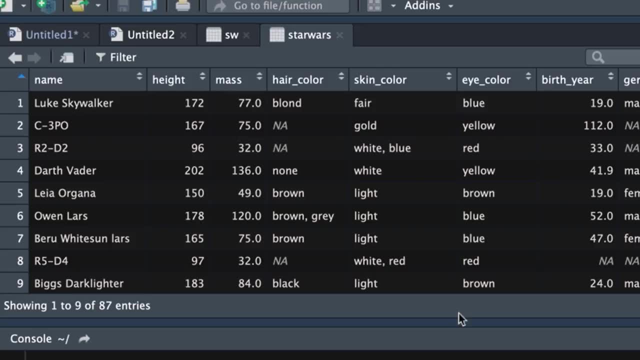 Today we're going to talk about how to recode data. Now, what do I mean by recoding data? Let's take a quick look at the Star Wars data set that's on the screen right now. So in the Star Wars data set which, incidentally, if you've installed the Tidyverse package onto- 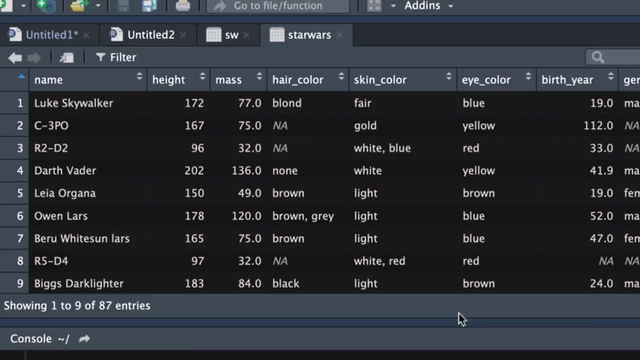 your computer. you've got this data set. you can practice everything I'm going to show you at home, Right? so the Star Wars data set's got rows which are Star Wars characters, Luke Skywalker, etc. etc. etc. and columns that are variables. we've got name, height, math, etc. etc. Now how, using our 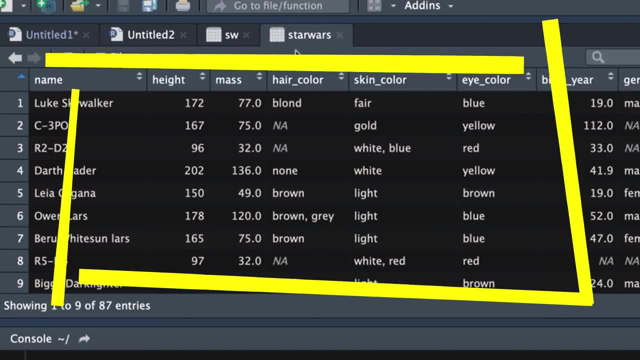 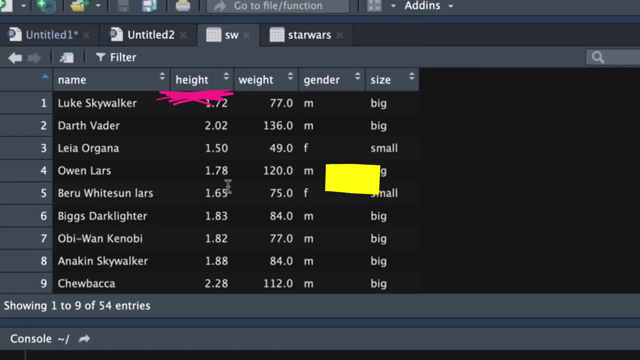 programming. do we get from this data set- the original one- into a new one that I'm going to create over here? that is a little bit different. Let me talk you through the differences right Here. we've got height in meters squared. The original data set had height in centimeters. 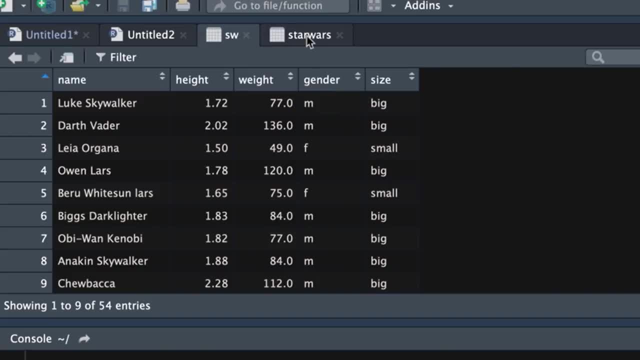 We've also got gender using m and f instead of in the original set we had male, female, etc. etc. Also, we've gotten rid of all the missing values. We've created a new variable called size: Characters that are big that meet the criteria of being taller than one meter. 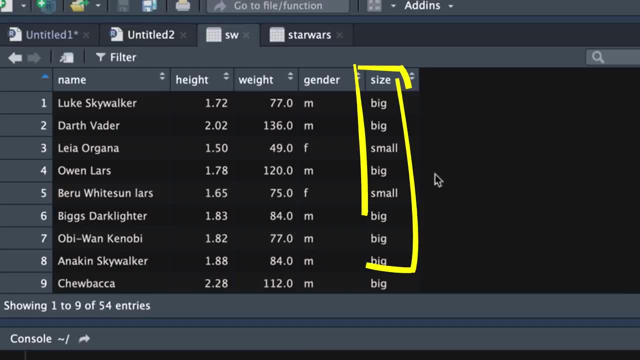 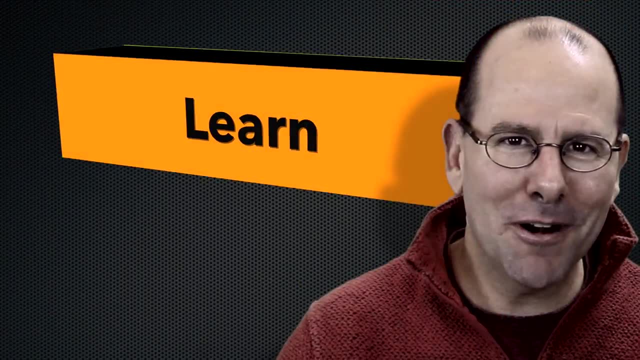 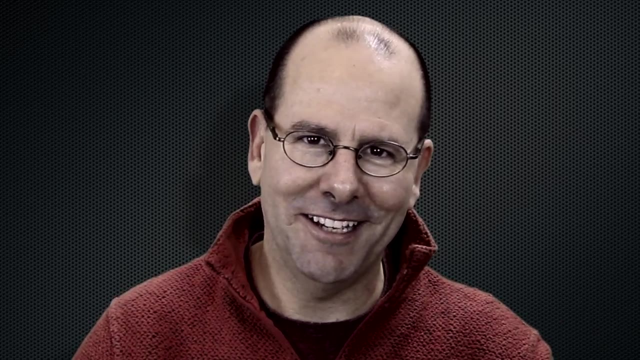 and weighing more than 75 kilograms. Right, so let's see how we can get to this new data set from the original one using some simple code. If you want to learn about R programming, then you have come to the right place. On this YouTube channel, we're creating R programming videos on everything.